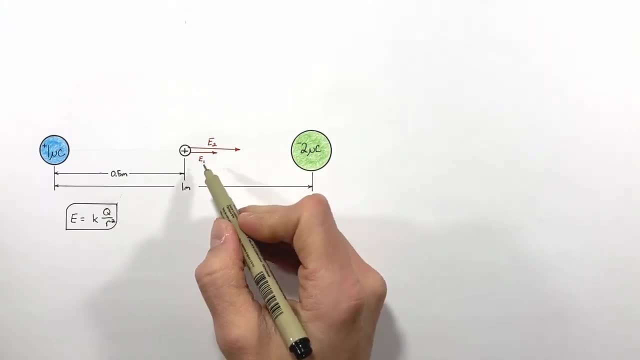 that the electric field from charge 2 and realize these electric fields are vectors. so we're simply going to add together these vectors in order to come up with the total electric field. so, applying our equation for electric field first to the field produced by this positive 1 microcoulomb charge, we find: 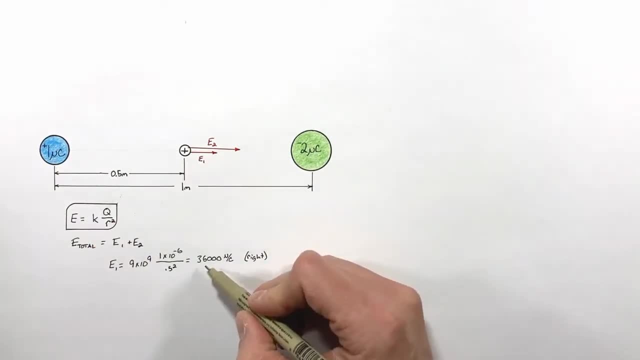 the electric field at this point produced by this charge is 36,000 Newtons per coulomb. that simply tells us that if we were to put a 1 coulomb test charge right here, there would be 36,000 Newtons of force acting on it. now 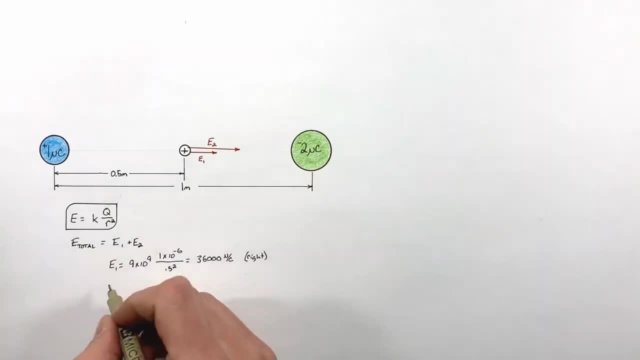 working out the electric field from this second charge. we find the electric field at this point from this negative 2 microcoulomb charge is 72,000 Newtons per coulomb. now you'll notice I didn't include the negative in my calculation here. the negatives and the positives can. 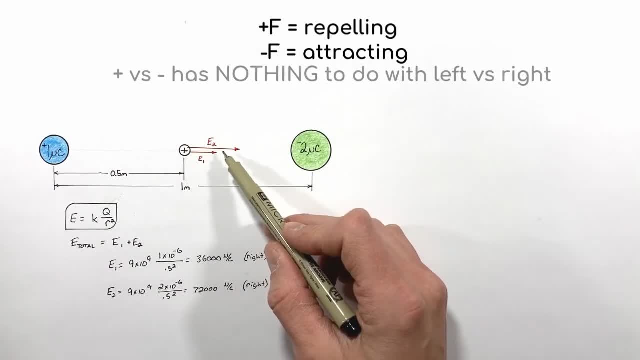 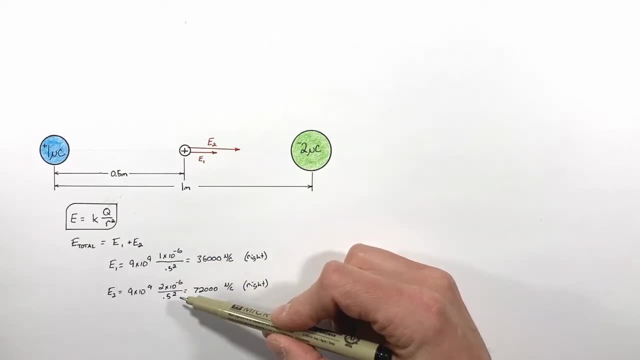 serve to help us understand the direction which a electric field is acting, but I find when you put it in the math it can become a bit confusing. what I prefer to do is leave the negatives and positives out of the calculations and simply determine their directions conceptually, like what we did here. but 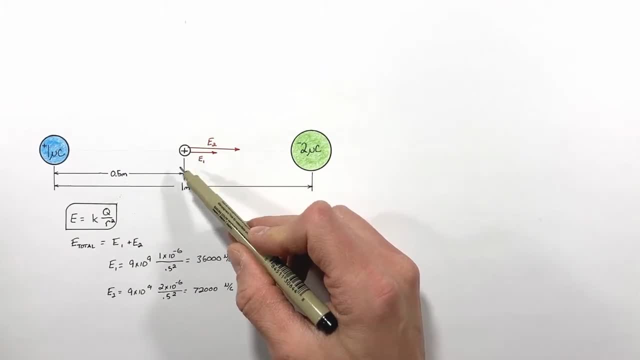 remember, we're trying to find the total electric field, which is going to be the sum of the two electric fields, and we find the total electric field at this point right here is 108,000 Newtons per coulomb. next I want to go through and work out the magnitude and direction. 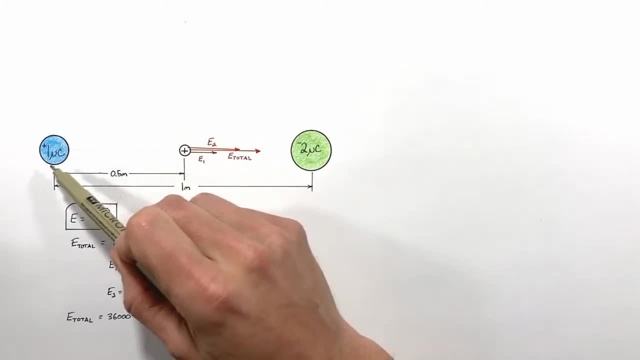 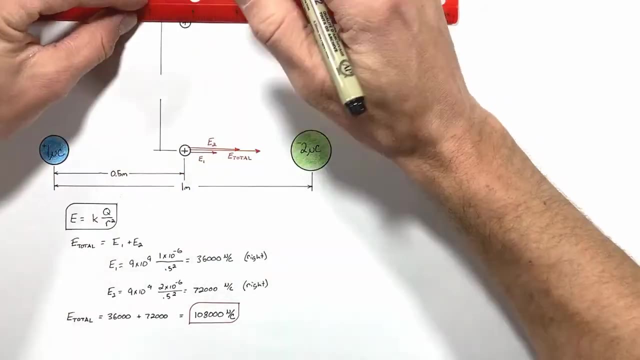 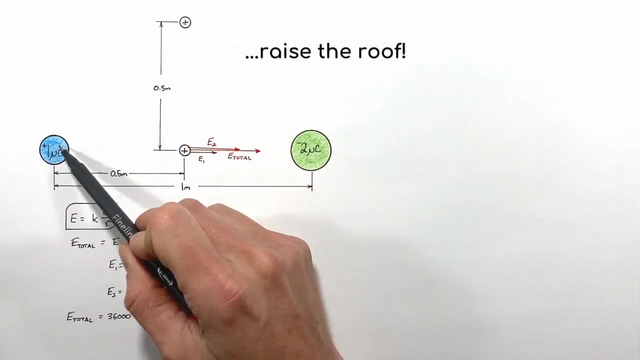 of the electric field at a point that is not nice and neatly centered between these two charges. because of coulombs law, positive test charge which is placed right here in our electric field is going to be pushed away from this one microcoulomb charge. 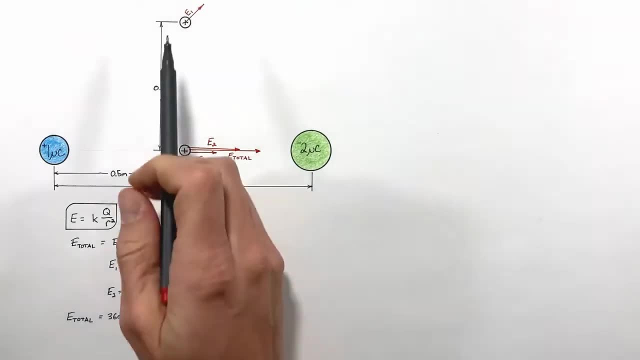 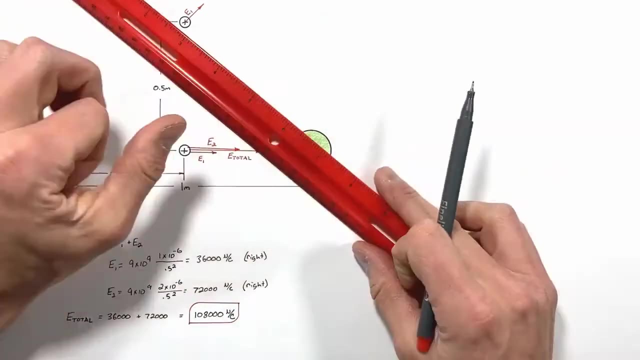 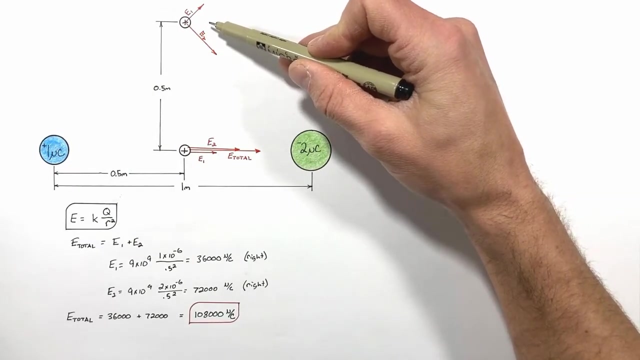 That will be up and to the right And this positive test charge placed right here will be pulled down and to the right towards this two microcoulomb charge. And in this problem we're going to solve for the total electric field And much like before, we're simply going to look. 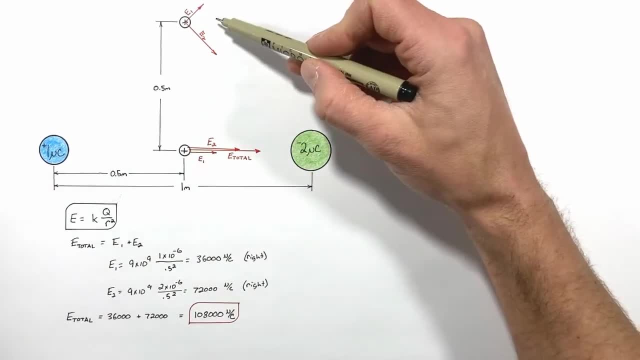 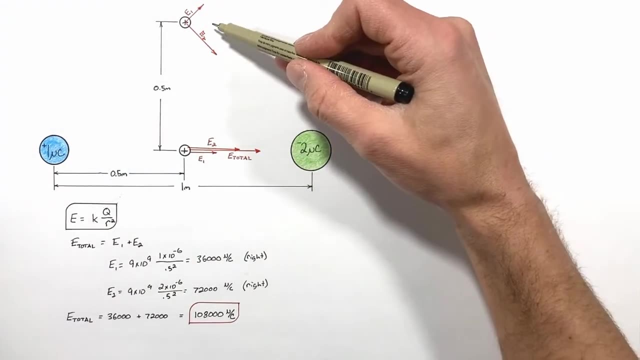 at the sum of these two electric fields. But remember, electric fields are a vector, So really all we're doing here is vector addition. So in order to find the sum of these two vectors, what we first need to do is come up with the magnitude. 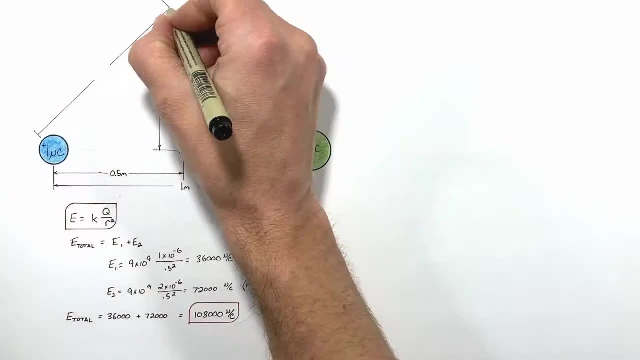 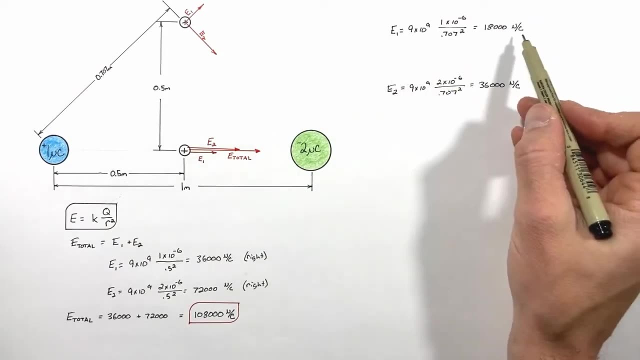 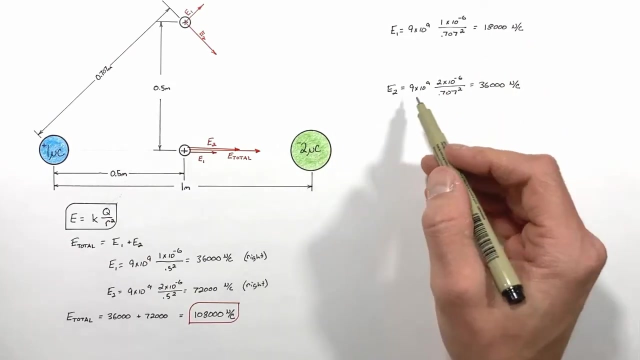 of each of these vectors And we find the electric field as a result of the one microcoulomb charge is 18,000 newtons per coulomb And the magnitude of the electric field from the two microcoulomb charge is 36,000 newtons per coulomb. 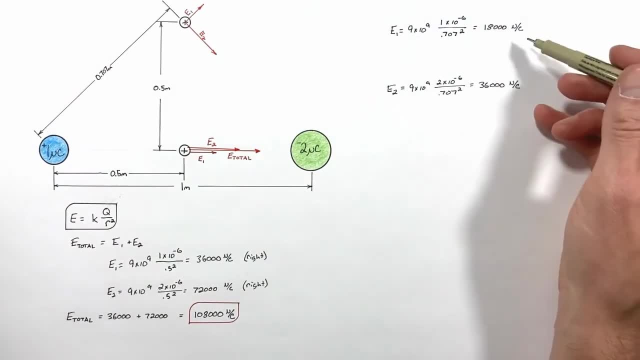 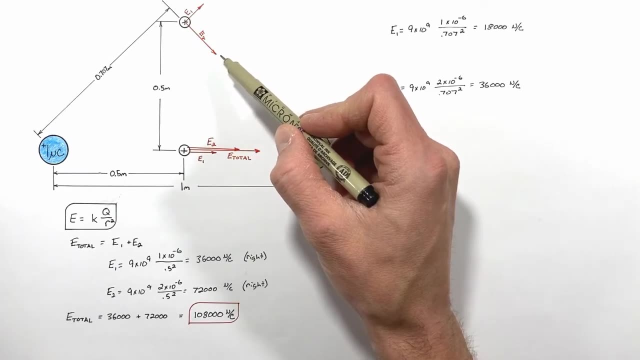 Now it's tempting to simply add together these two magnitudes, But remember, we're dealing with vector addition here, where we have a vector that's up and to the right and a vector that's down and to the right. So in order to add these two vectors, 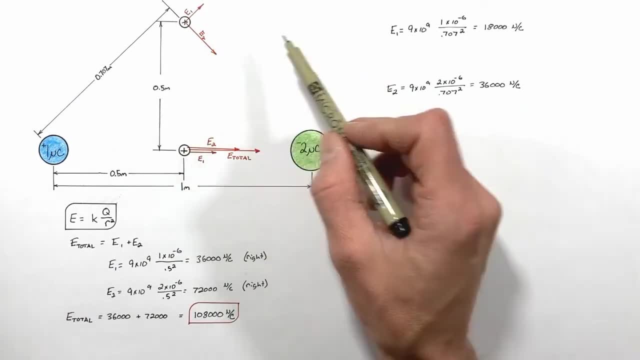 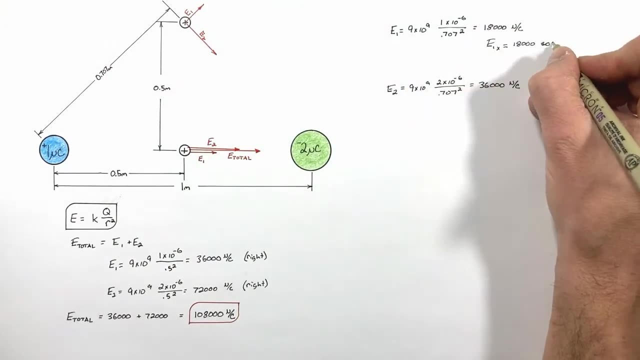 we're going to need to break these vectors up into their magnitudes in each axis and then add them together. Now, remember, we have to be a little bit careful when doing vector addition, because we don't want to lose the magnitude of each of these vectors. 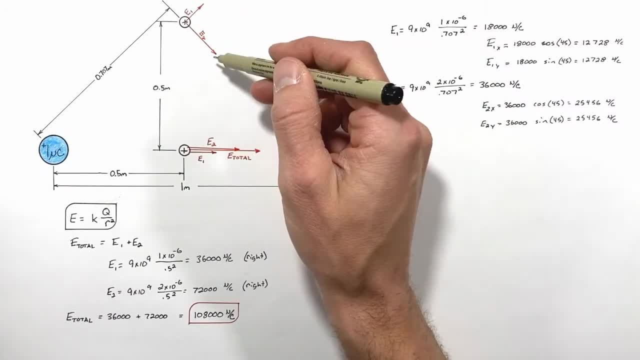 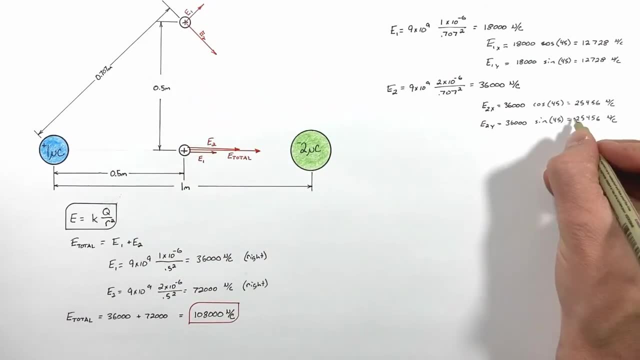 We want to be careful when doing vector addition because the vertical components here are in opposite directions. So I'm going to go ahead and say the vertical components that are up are positive and down are negative. That means this term right here is negative. So in coming up with our total electric field horizontally, 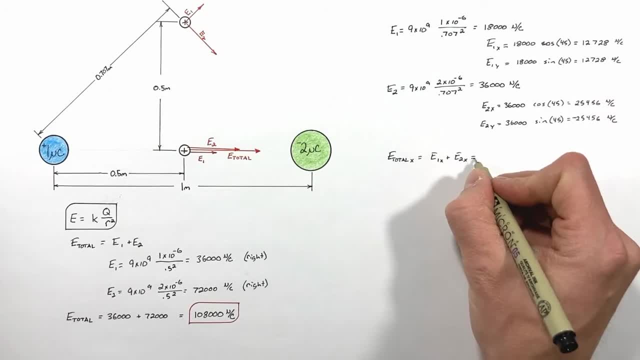 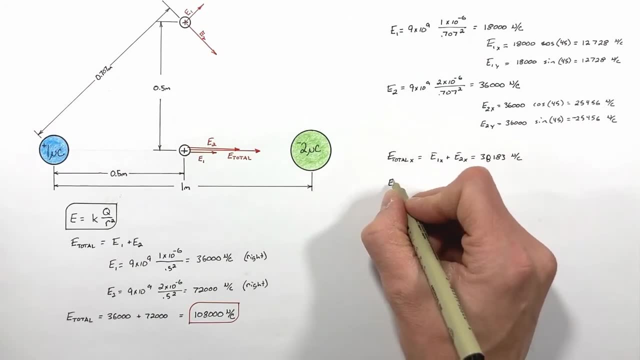 we're simply going to add together the two horizontal components. We come up with 38,183 newtons per coulomb And vertically, we're going to add together the two horizontal components And vertically, we're going to add together the two horizontal components. 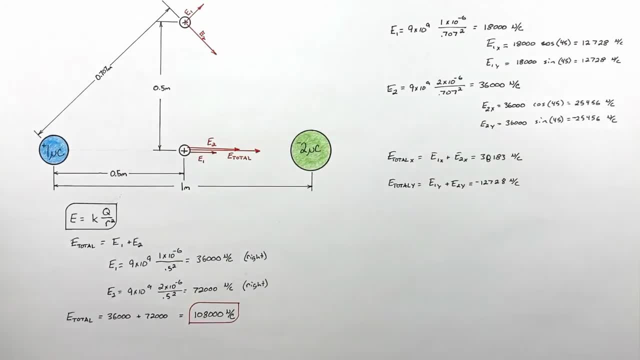 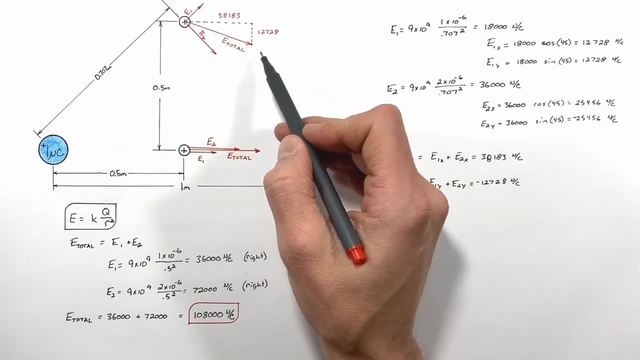 We come up with negative 12,728 newtons per coulomb. We come up with negative 12,728 newtons per coulomb. So, knowing the components of our total electric field, we can now solve for the magnitude of the total electric field. 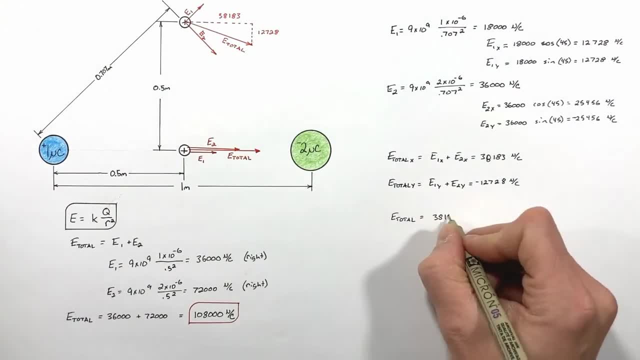 using the Pythagorean Theorem, We find the electric field at this point has a magnitude of 40,248 newtons per coulomb. has a magnitude of 40,248 newtons per coulomb. And to find the direction of the electric field,